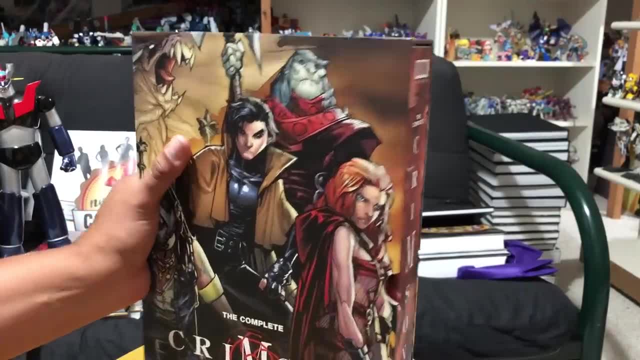 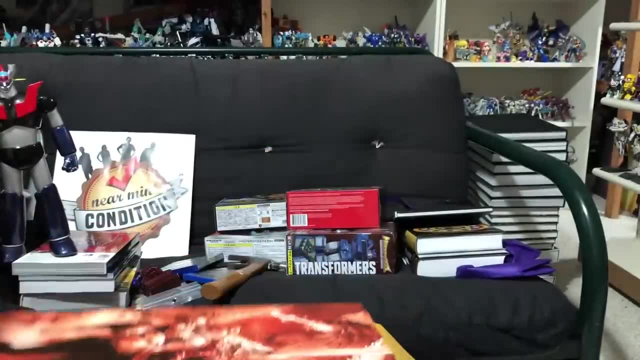 Alright, let's take a look inside of this book, And please excuse the mess, as I'm doing some reorganization down here in the basement, moving all my collected editions here. Um so let's look at the slipcase. It's really nice. 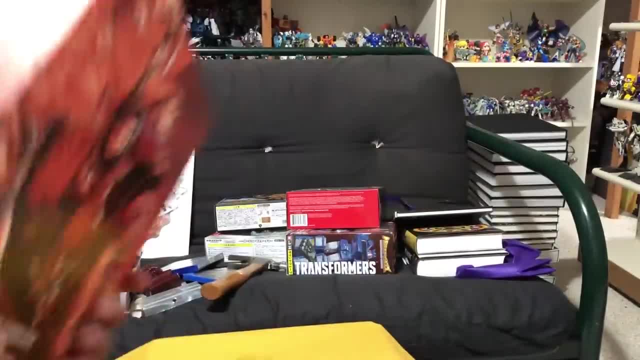 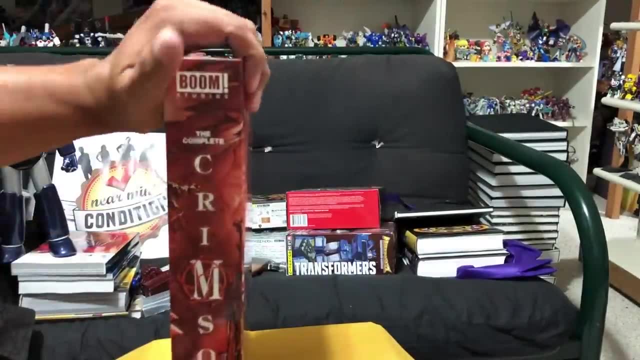 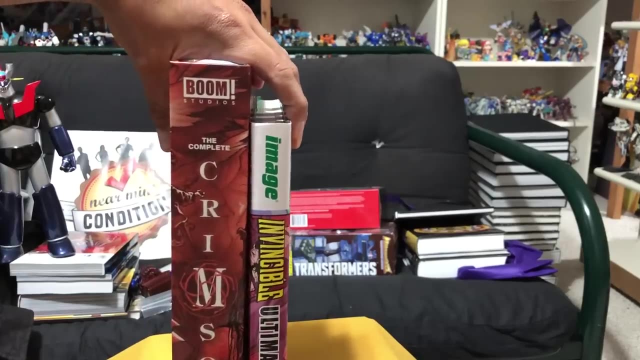 Looks like one of those Absolute slipcases. And this is what the inside of the book looks like. It's got a red crimson color to it And as far as size and height let's see, compare it to an OHC. This is Invincible by Image Comics. 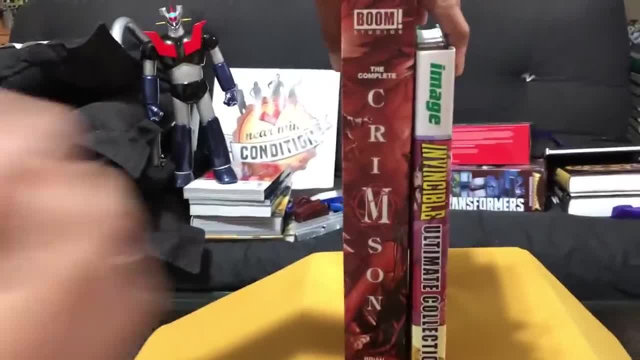 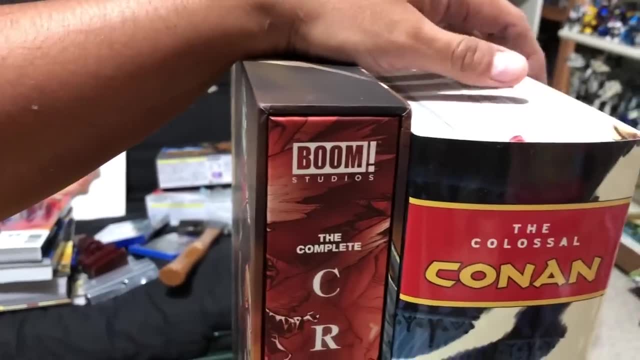 And you can tell a little bit of the size there And let's look over here at the dimensions. So it's a little bit bigger And just really quick in the box. I wanted to compare it to the size of an omnibus. 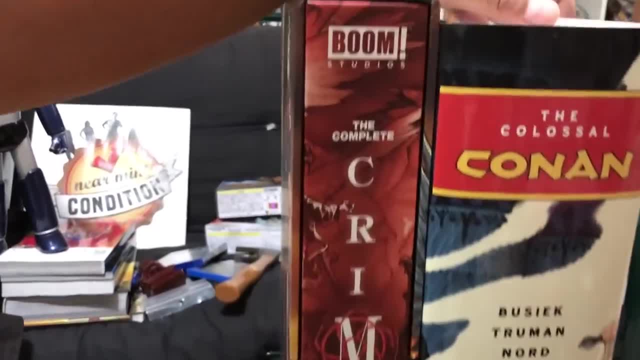 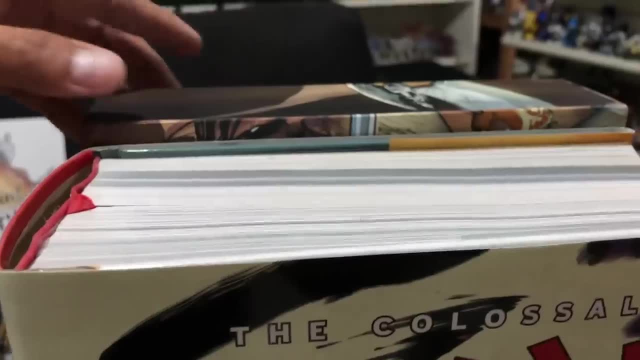 It is the Colossal Conan right there. It's just a tad bit taller, not too much, And out of the box it's just a smidge taller, but you can't really tell that much difference. You can tell a little bit more from there. 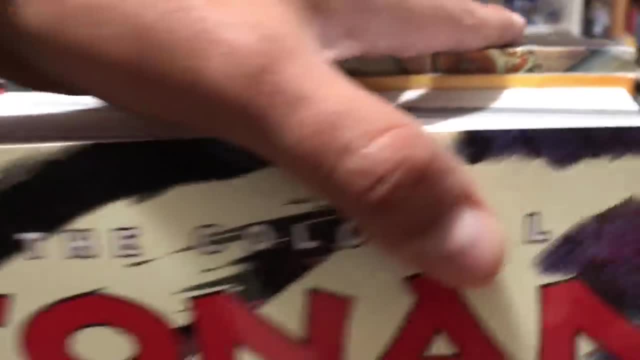 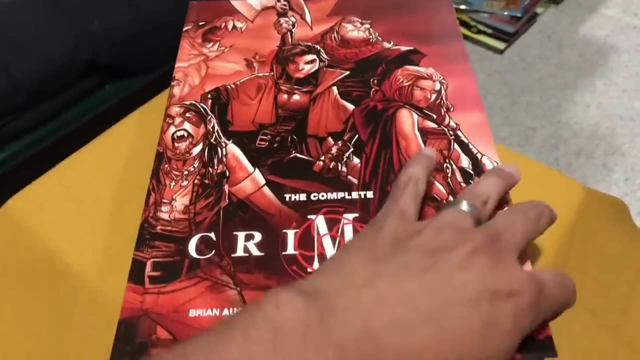 Um, Maybe just a little bit longer, Not too much, though. Now let's look inside and talk just a little bit about the book. I wanted to go ahead and do a little overview of this in case you didn't know what it was or were on the fence of buying it. 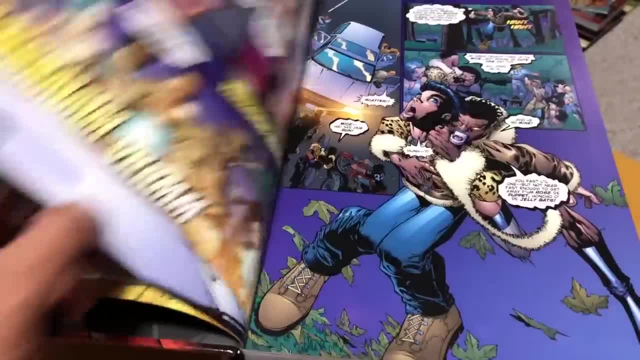 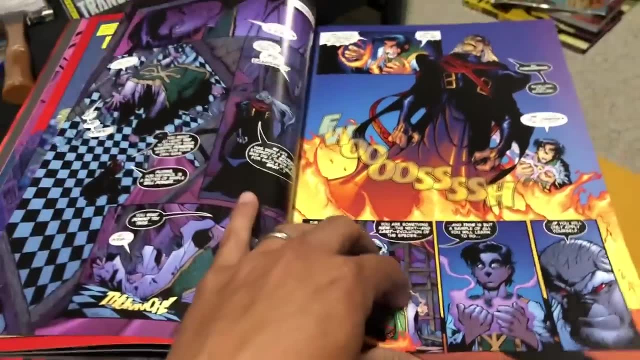 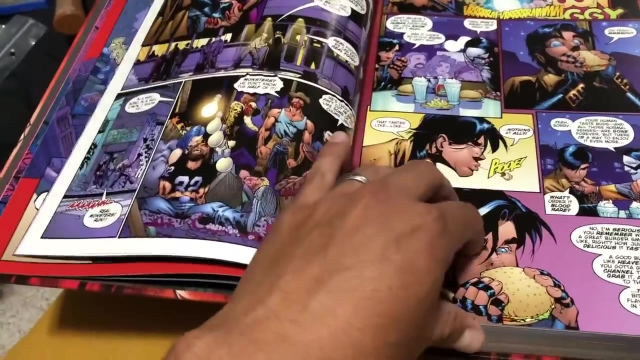 The story is mainly by Humberto Ramos and two of his other friends, And the script is written by Brian Augustine. So this complete collection collects Crimson 1-24, the half-issue, the source book and then the- I think it's- the Scarlet XX miniseries. 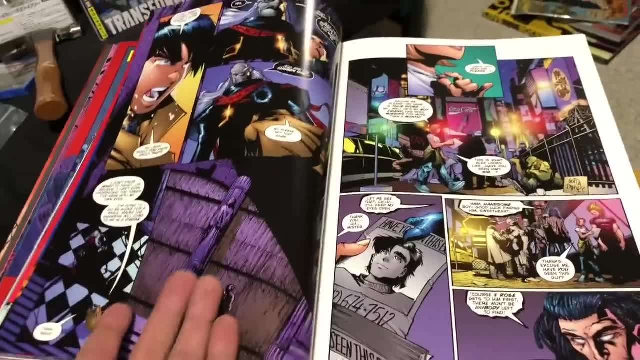 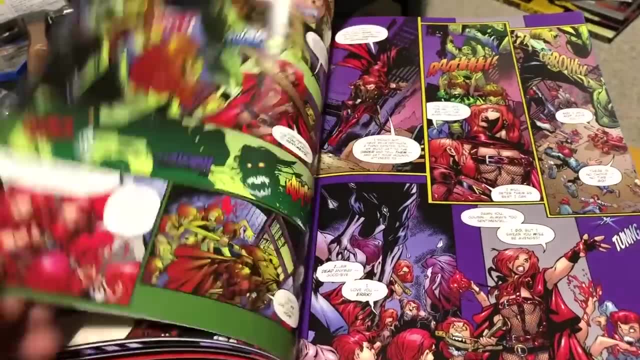 Not a miniseries. I'm sorry, it's a one-shot. Um, I don't remember much about this book. honestly, This is at the time when I stopped reading comic books, but my brother was huge into this stuff. If I'm not mistaken, I think it was Cliffhanger Studios that did this. 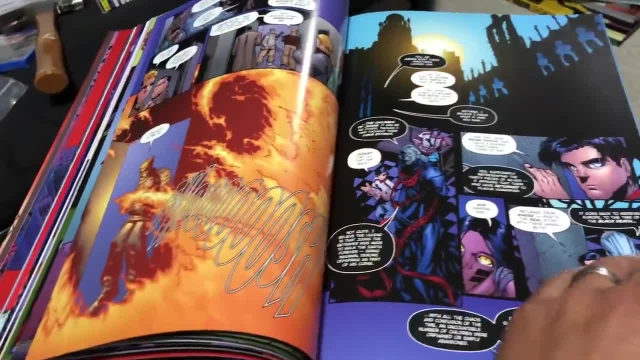 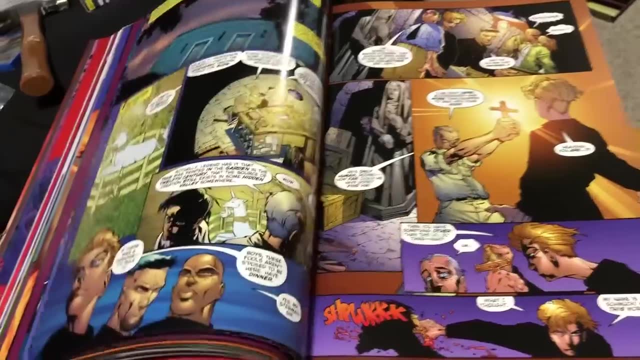 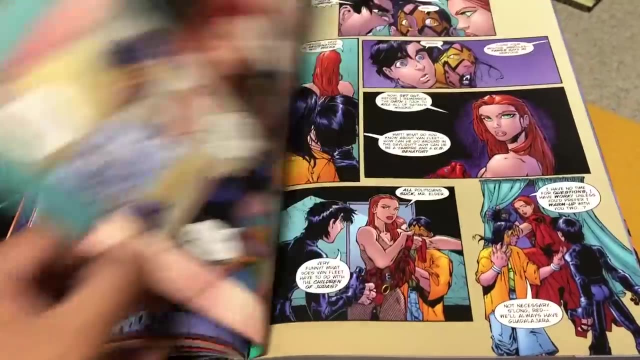 The same studios from Image that did Battle Chasers and also did Jeff Matsuda's Kaboom, if I'm not mistaken. So my brother would love to have this And Kaboom as well. I bought this as a blind buy when it was on pre-order from Amazon for $30. 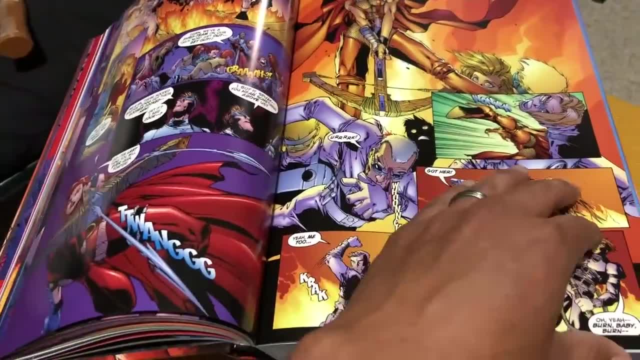 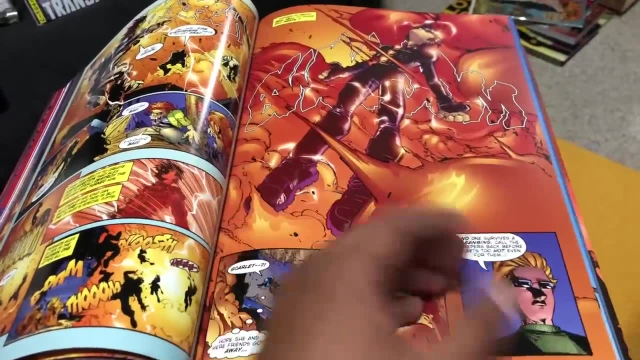 I guess it was a glitch, because the book retails for about a hundred and something dollars right now. I think they are completely sold out, but you can still get them through in-stock trades. So if you're a fan of Humberto Ramos, this is his baby. 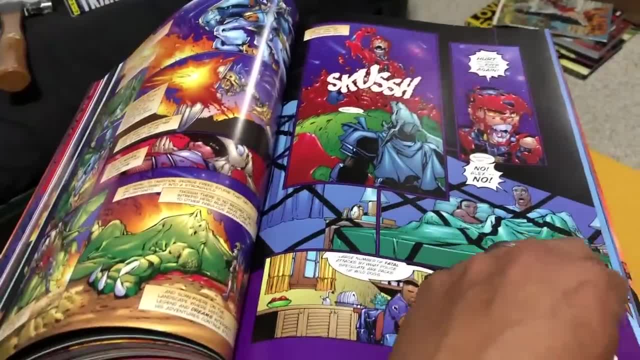 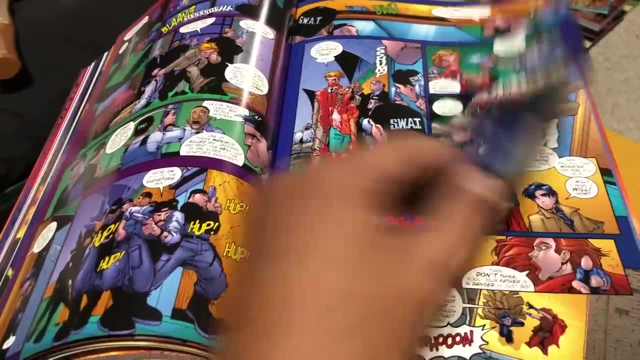 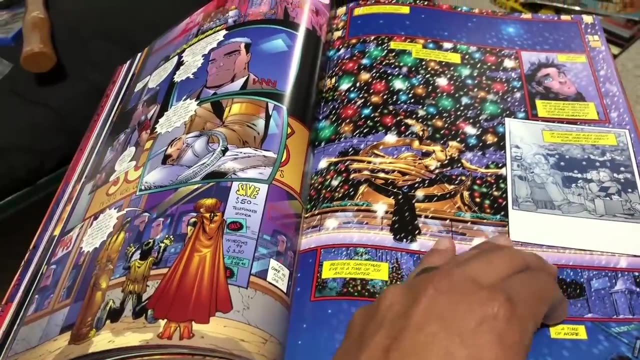 This is his art from the 90s. I remember first seeing his stuff- He had a very anime-ish look to his stuff. Uh, He was doing Impulse. and then Nation X, which was the short-lived 2099 series Or X. 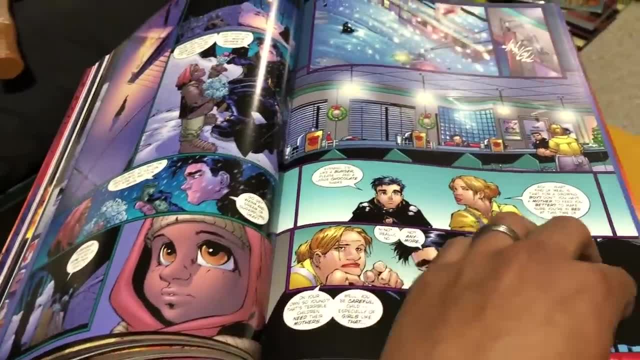 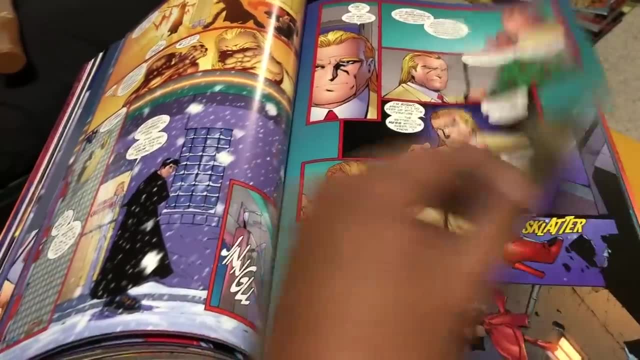 No, it was called X Nation, I'm sorry. X Nation 2099.. I remember that series from Marvel And then, of course, his long run on Amazing Spider-Man. Some people hit or miss for them, but I really enjoy his anime-ish art style. 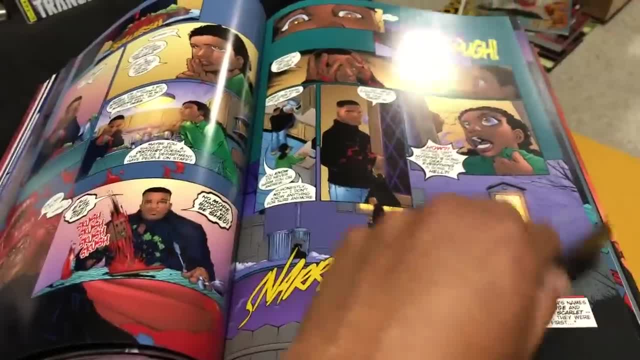 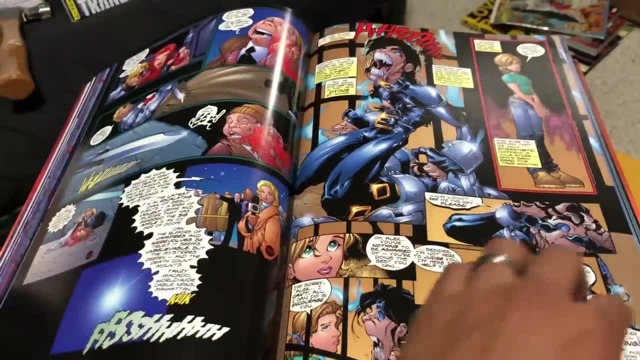 So the story, as you can probably tell as I'm flipping through these pages here, is about Alex, this young protagonist who is one of the last vampires- He's known as the Chosen One, And there's a huge war about to break. 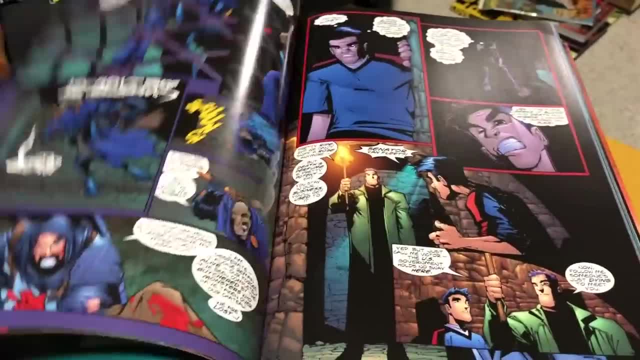 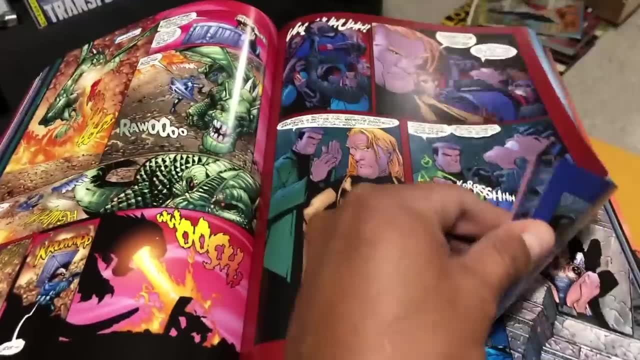 That's all I really know. I mainly got this because of the art, Because, like I mentioned earlier, I'm a huge Humberto Ramos fan. I like the colors. Some of the ink is done by Sandra Hope, who went on to ink some of Jim Lee's work. 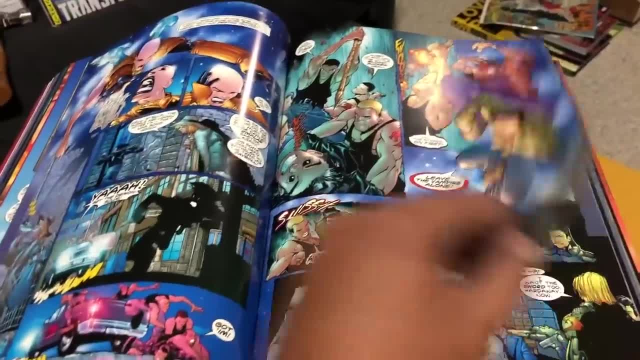 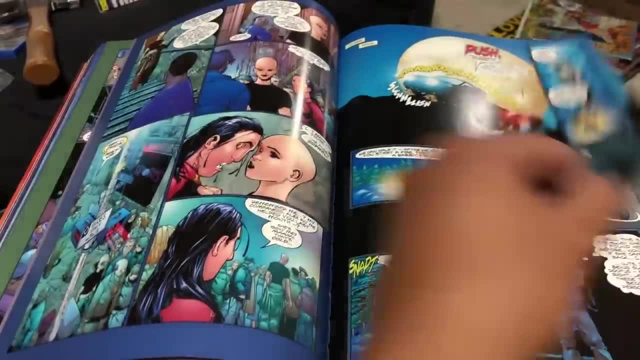 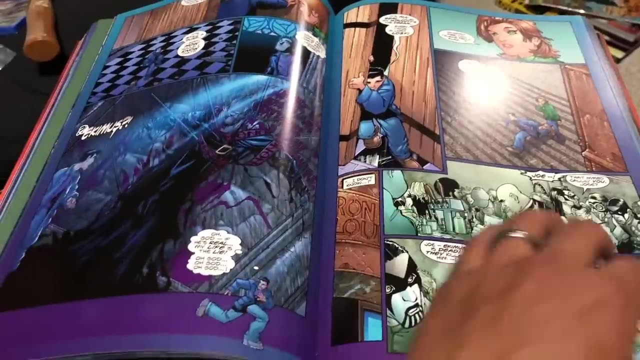 Especially on covers during Infinite Crisis. And, as I mentioned before, Brian Augustine did the main script- And if that name is familiar at all to you, it's because he and Mark Waid teamed up together on Flash- And then he was an editor, I think, during the late 80s, early 90s at DC. 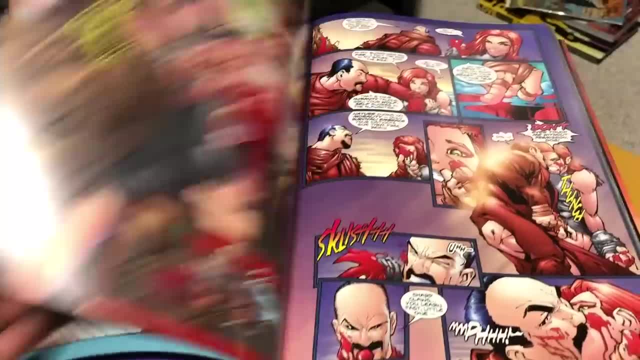 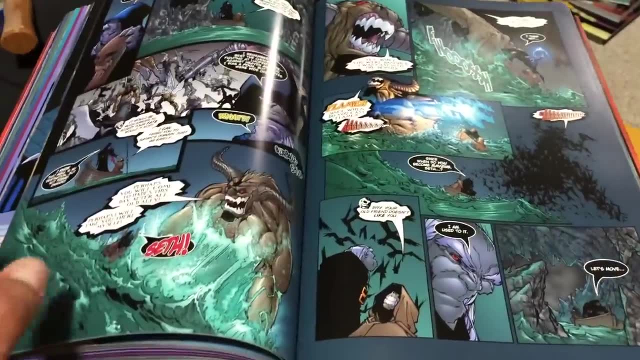 And he went on to do yeah Flash. So he had a pretty big run there with Mark Waid. So he just did the script, The main plot and all that, like I said, is done by Humberto Ramos And actually I want to go ahead and give credit to his title. 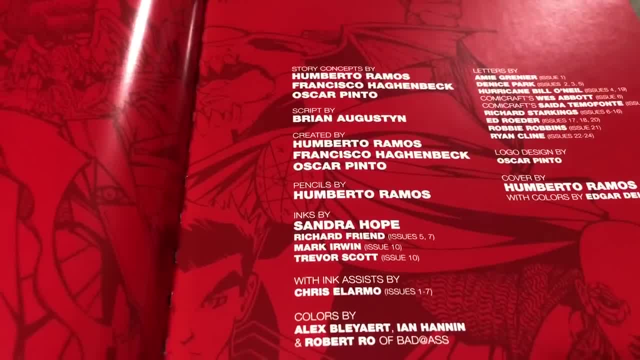 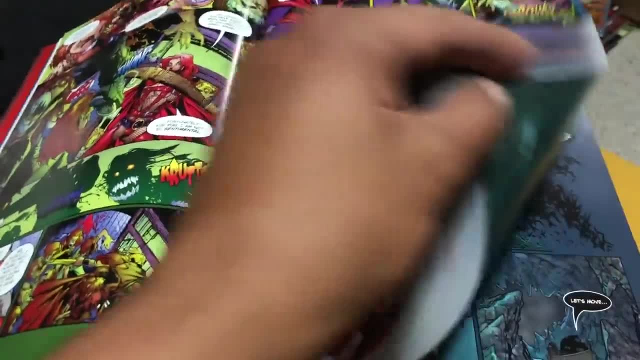 To his two other friends. It is Humberto Ramos and Francisco Hagenbeck and Oscar Pinto. Those are the guys that created the book and the story concepts behind it. Let's flip through it here. It's got that 90s. look to it. 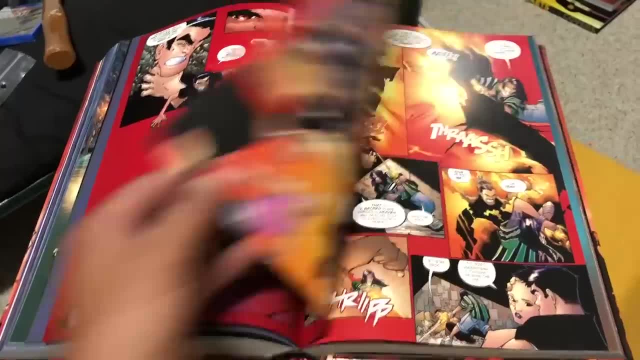 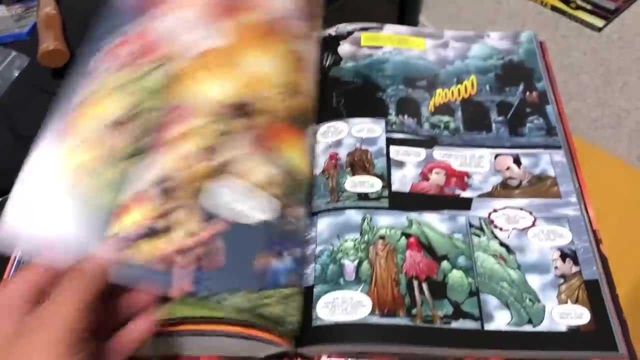 It reminds me a little bit of, like I said, Battle Chasers or Kaboom, Which all came from the Cliffhanger line Which also had the Gen 13 and Danger Girl by Jeffrey Scott Campbell. I have no idea if the story is any good. 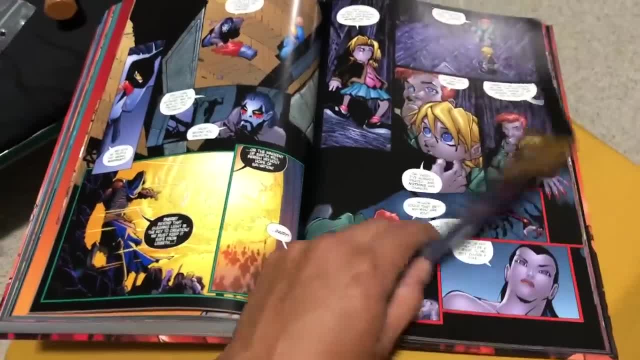 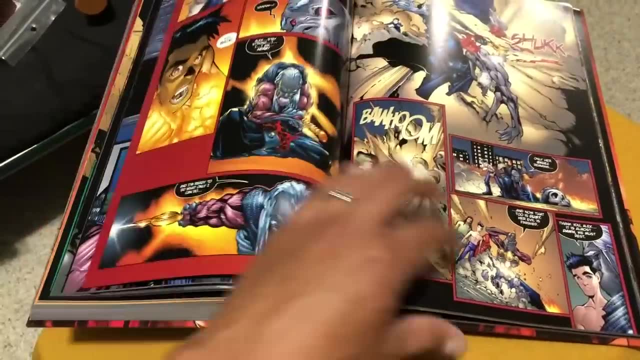 I'm just going to flip through it and look at the art, But as a blind $30 buy, that was okay with me. I'm not sure if I would pay $100 for it though, Unless you're a huge Humberto Ramos fan. 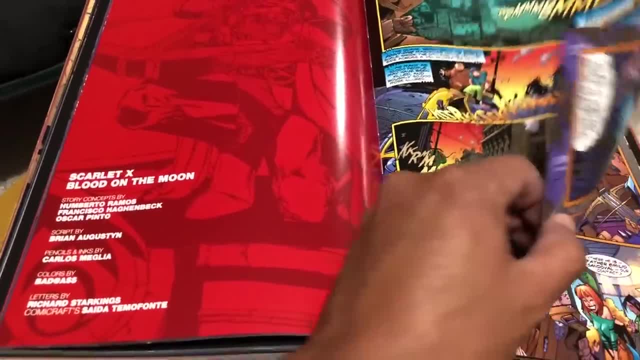 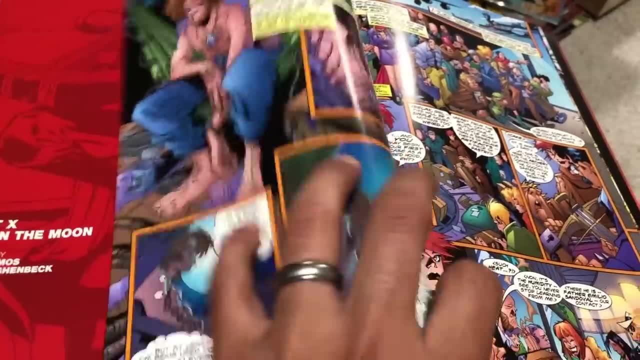 Okay, let's flip here. This is the Scarlet X, So it is just one X. Blood on the Moon, one shot. This one is actually not drawn by Humberto Ramos, But it is drawn by Carlos Meglia, But the story and stuff is still by him. 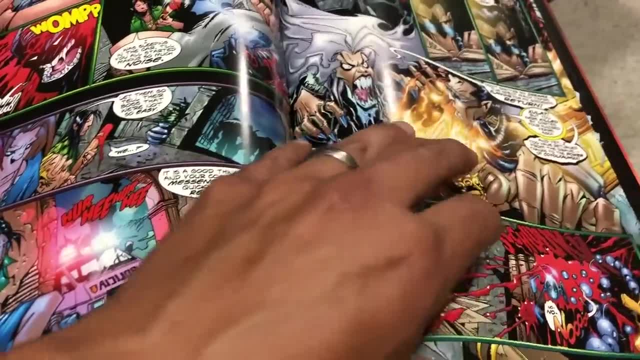 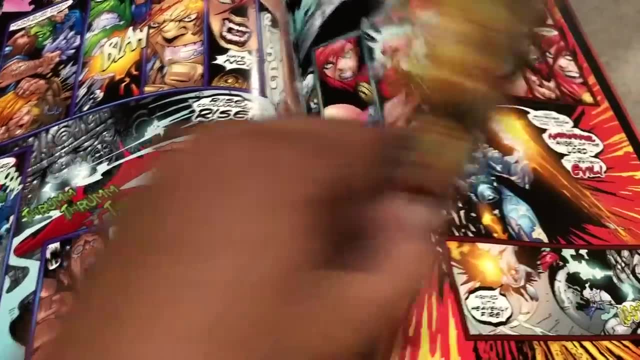 Now it was funny. I met Humberto Ramos, probably about during his Spectacular Spider-Man run. I'd say it was a little over 10 years ago And he didn't speak English, So a lot of the stuff had to be translated when I saw people in line. 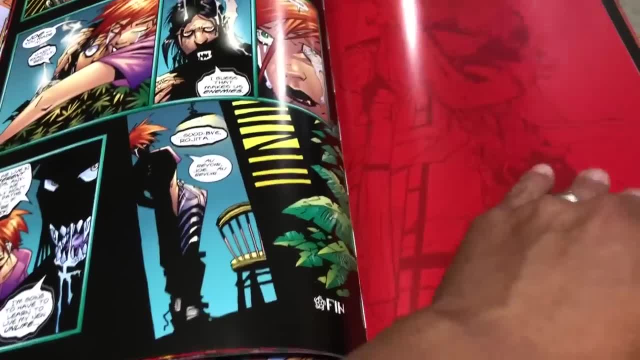 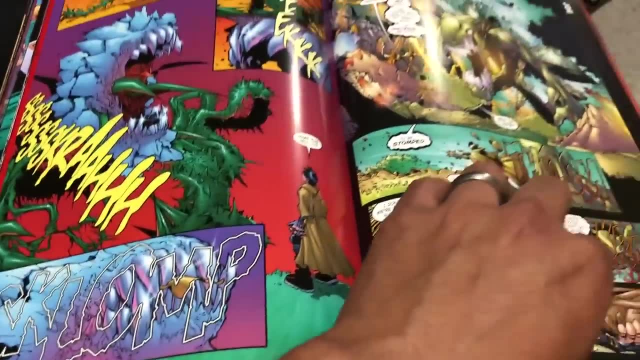 But I was able to approach him in Spanish and get him to sign a couple of my books. So there's that. Here's Crimson Half. This is drawn by Humberto Ramos. There was another book that I really liked that he did. It was called Revelations with Paul Jenkins. 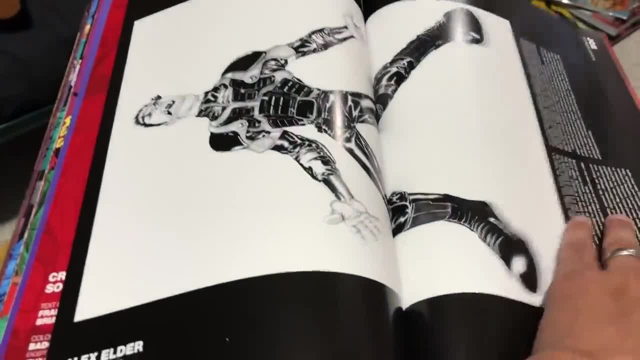 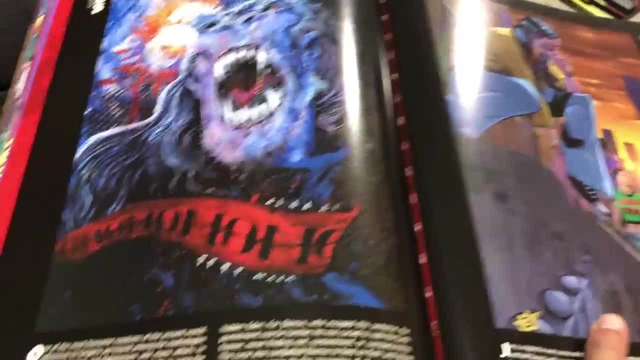 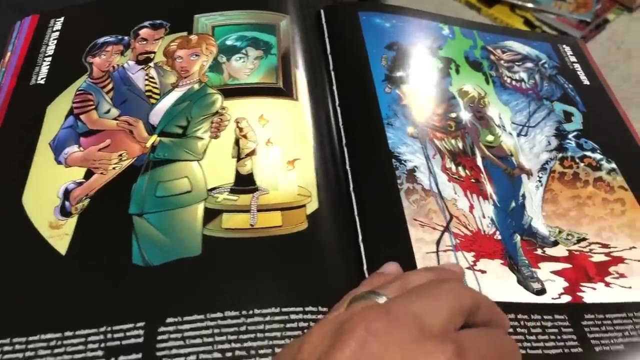 Because they both worked together on Spectacular Spider-Man. This is the Crimson Sourcebook. Really really liked that picture. Looks like it's just pictures by different artists. Looks like David Mack, But just your typical Wildstorm sourcebooks. Yeah, now the license belongs to Boom. 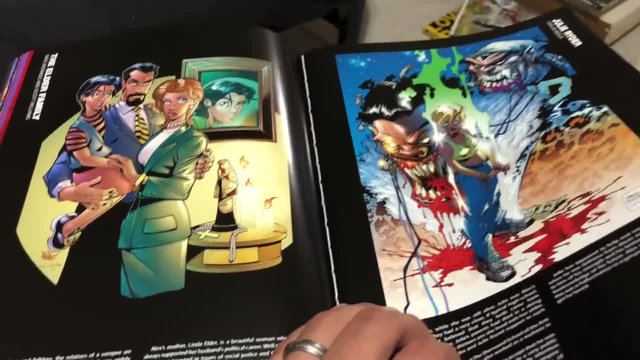 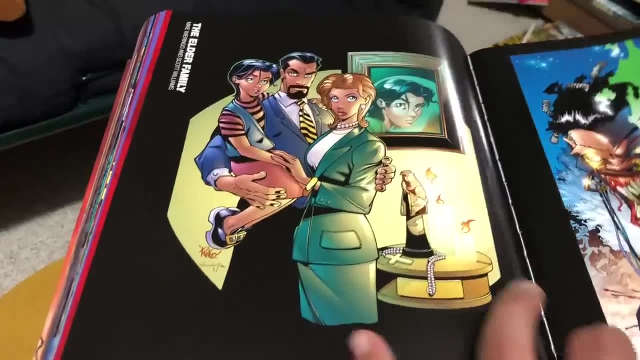 Guess it went from Cliffhanger to Wildstorm to Boom Comics. That looks like Jeff Matsuda actually, But it's not. It's called Meglia. That's Mike Laringo, though Mike Laringo, That was the other book. 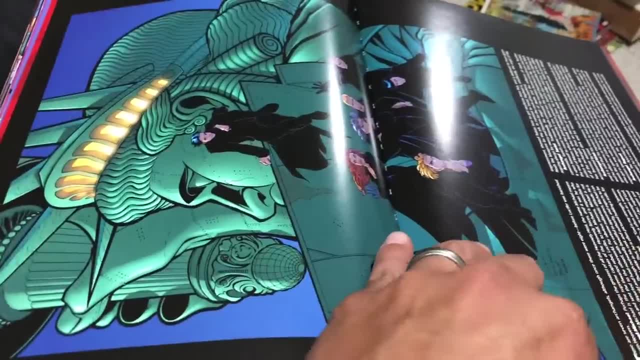 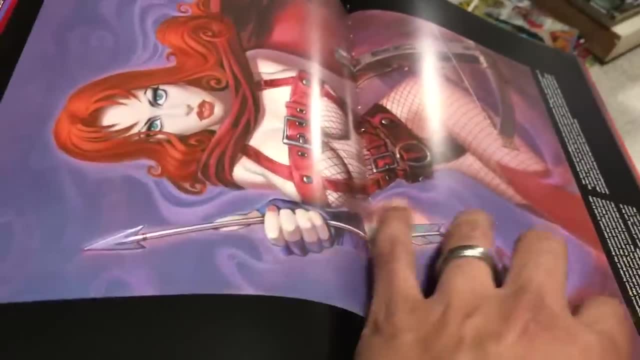 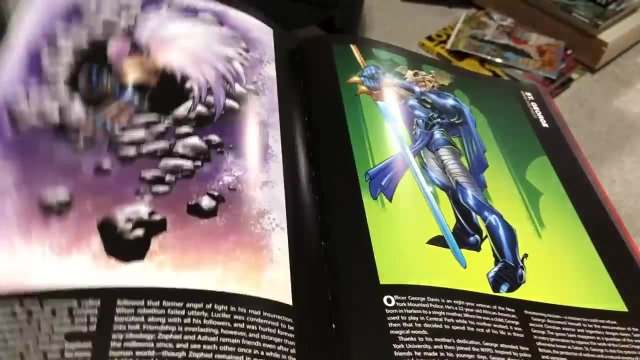 Telos. That was the book that he did. That's Mike Mignola. Yeah, Sourcebook is nothing, but That's really cool. That's Joe Chiodo. That's Scarlett. That kind of looks like Travis Cheris.